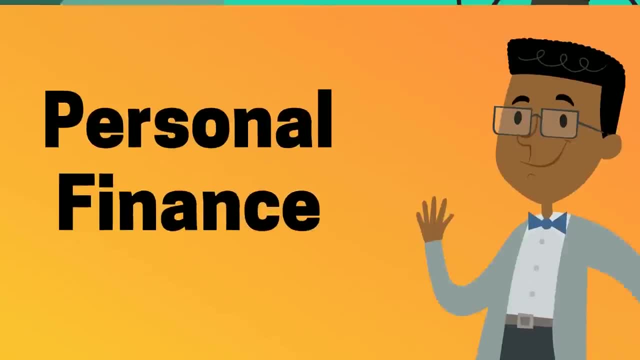 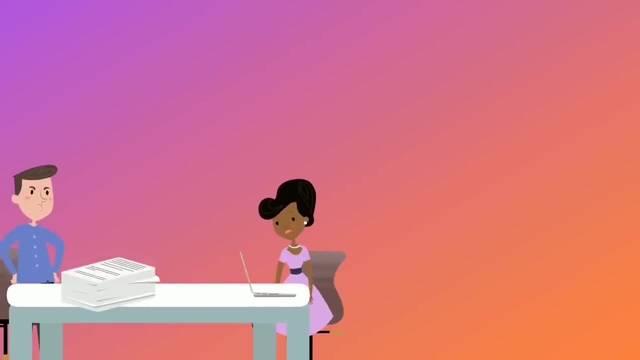 world, you need to know a lot more about money than what school will ever give you. Personal finance forms the backbone for all success stories. To save you from the hustle and bustle of having to learn from your mistakes, our team of experts have compiled a list of 10 most important rules that everyone should abide by. 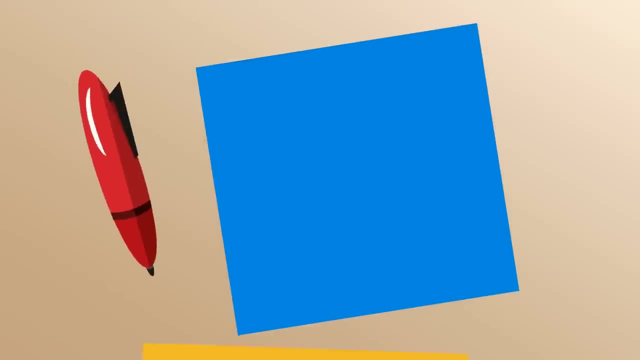 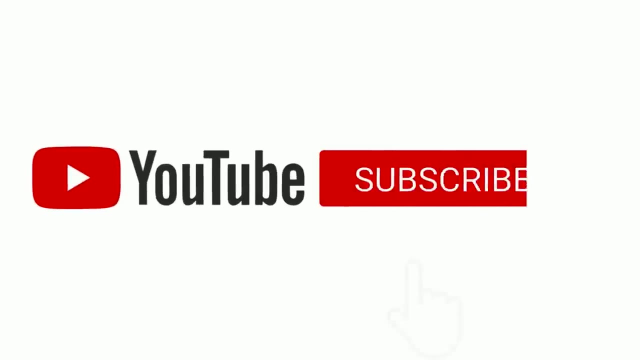 to be ahead of the game with their finances. Grab a pen and paper. Here are 10 of the most important personal financial rules you will never learn in school. Before we start, why don't you hit the subscribe button and the bell notification icon so you never miss any of our videos? Let's begin. 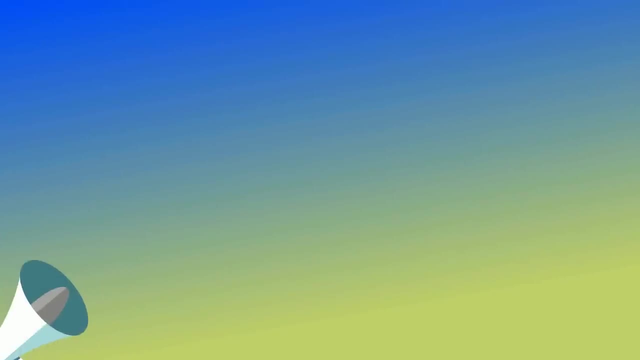 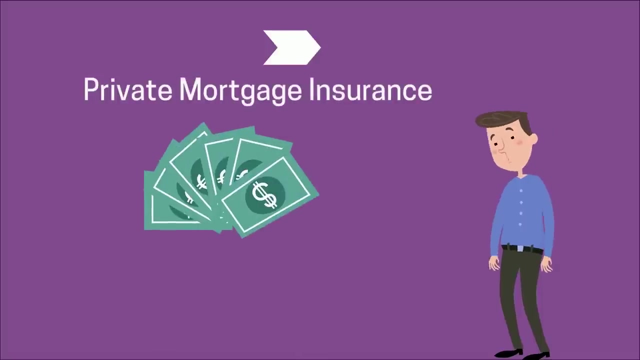 10. Buying Your First Home. You probably heard of the popular statement: if you want to buy a home, you have to save up to 20% of the value for down payment. If you don't, you'll be forced to pay private mortgage insurance. 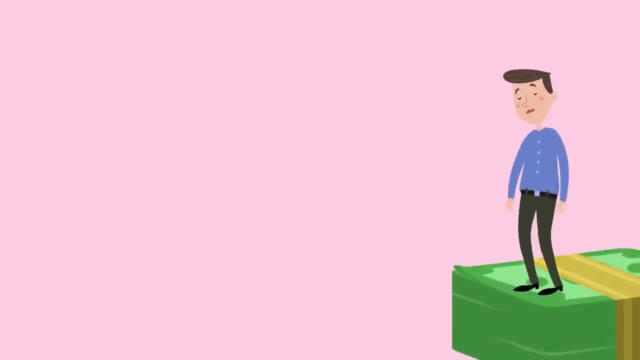 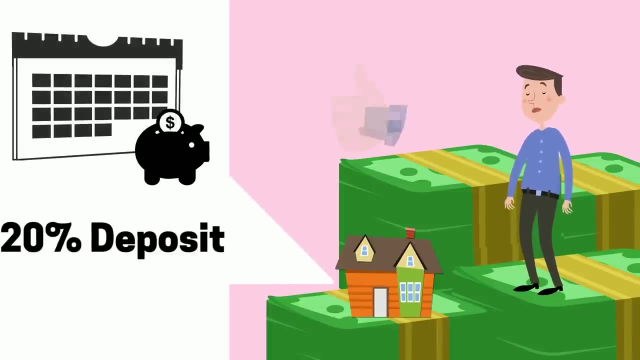 which could really dent your account. What you won't learn in school is that, while higher mortgage payments may be painful, the financial trade-off between paying more money now and waiting to save up the 20% deposit could be worthwhile When we look at the macroeconomic. 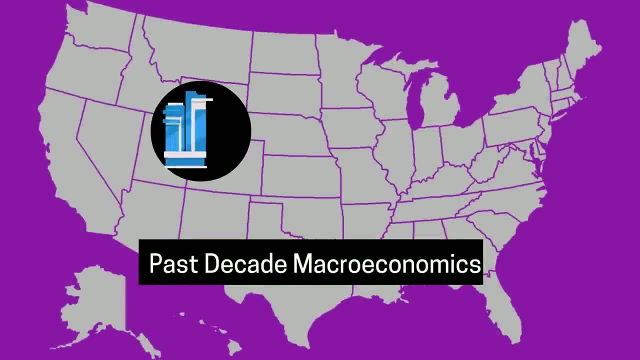 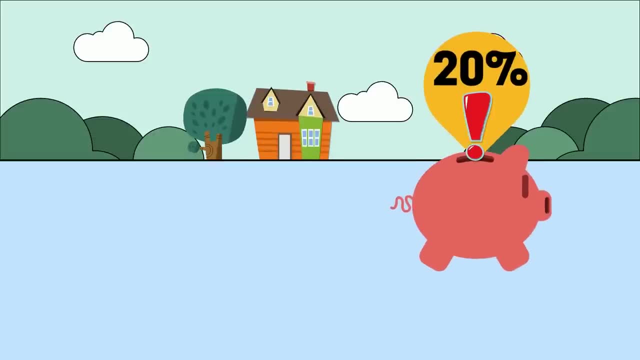 factors. in the US over the past decade the appreciation rate of real estate has really gone up, but the wage levels have remained stagnant. So it makes it unrealistic to start saving up 20% of the home value, as it will only increase drastically over the years. 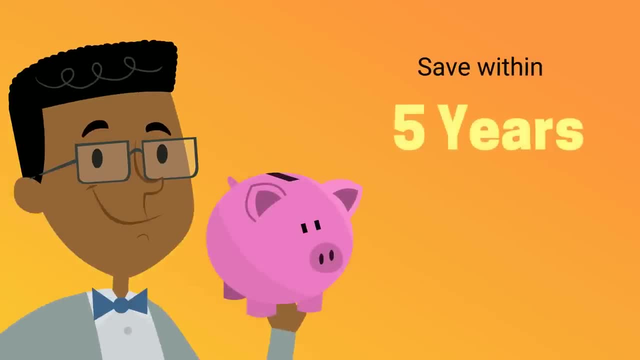 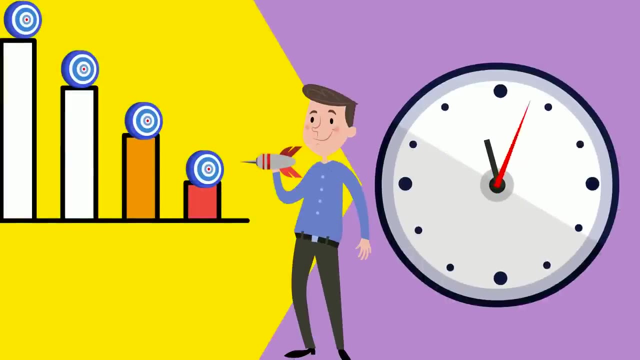 The rule behind this is: if you have the capacity to save the money within at least five years comfortably, then go for it. If you don't have the capacity to save up to 20%, then go for it, But if If it will take you longer, you will be chasing a moving target as the price increases. 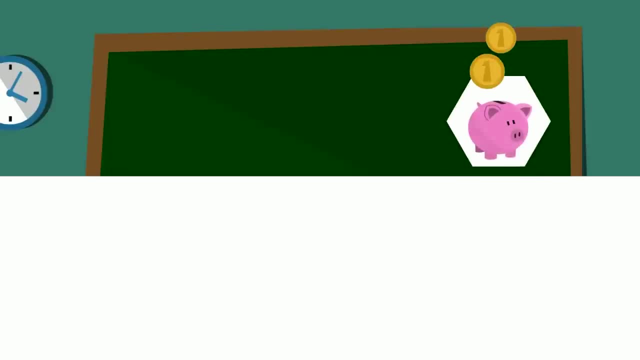 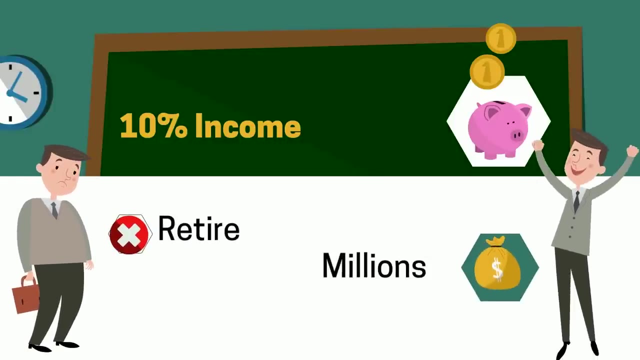 9. Save, save, save. In school, they will teach you to have at least 10% of your income. but let's be honest here. this isn't enough to retire on Well, unless you are earning millions. For most of us with a regular paycheck, a decent savings percentage will be about 25-40%. 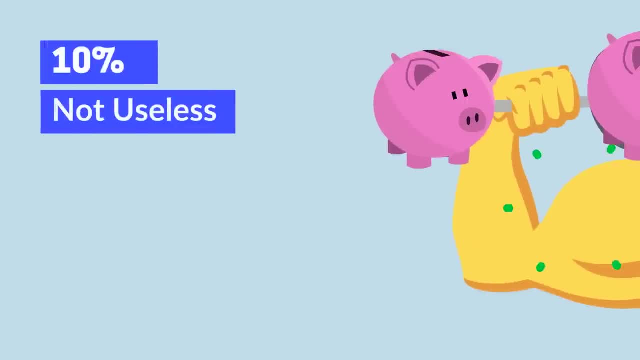 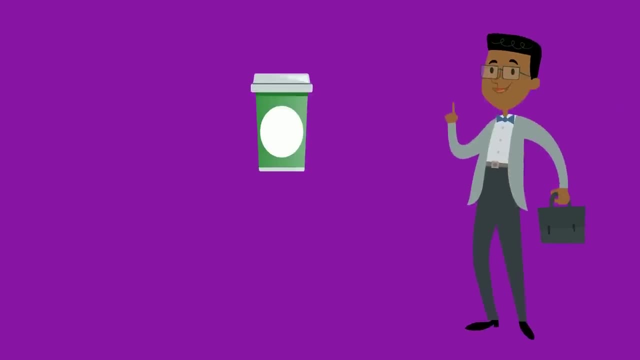 We are not saying 10% is entirely useless. it could be a great starting point to build that savings muscle In order to save more. reduce your expenses and unnecessary costs. Instead of buying that cup of coffee every morning, put that money in a savings account. 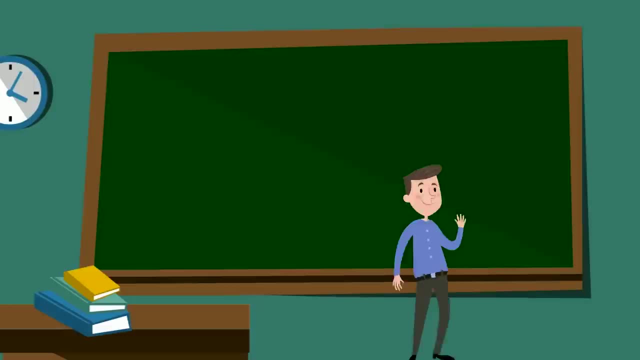 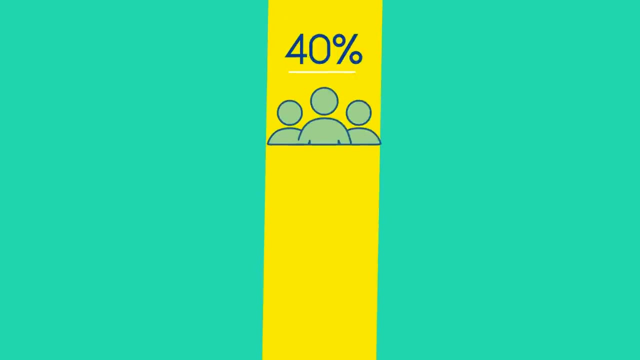 with a better interest rate. 8. Emergency Fund. You may have never heard of an emergency fund from school, but you are lucky. you have us to teach you about it. Recent statistics show that up to 40% of Americans don't have the funds to cover an emergency. 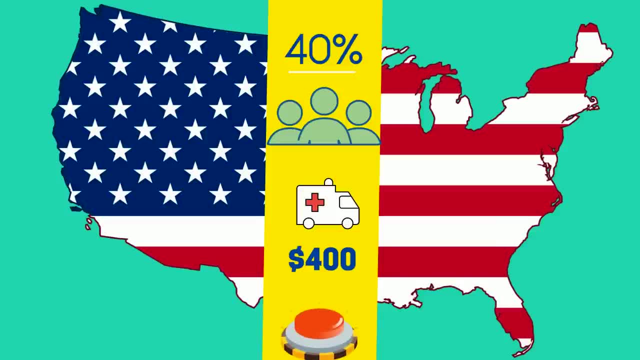 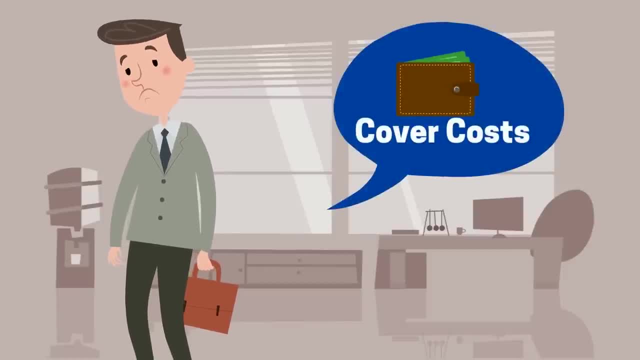 of $400.. This is an alarming statistic that only shows how people disregard the importance of an emergency fund. What if you lost your job today? Would you have enough money to cover your costs? The golden rule is to have 6 months of expenses saved up somewhere, but we suggest that if 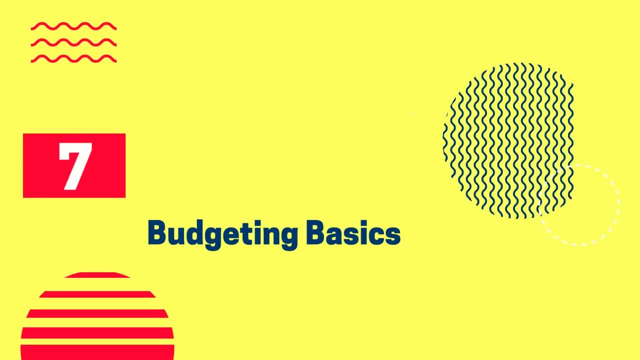 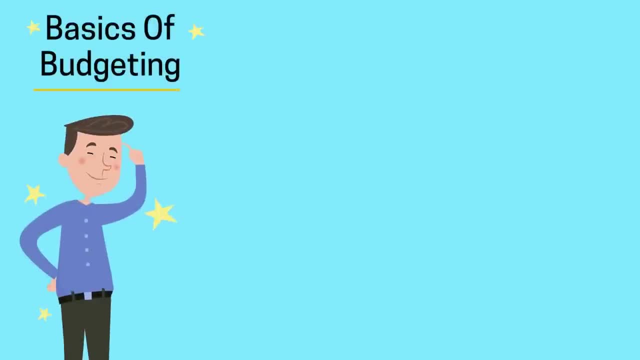 you can make it more the better. 7. Budgeting Basics. Budgeting is quite important in life, yet you won't hear anything about it in school. Sadly, not understanding the basics of budgeting while in school can leave you disadvantaged right after graduating, especially once you move out. 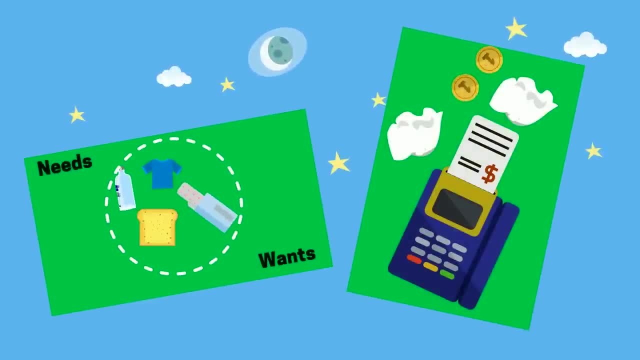 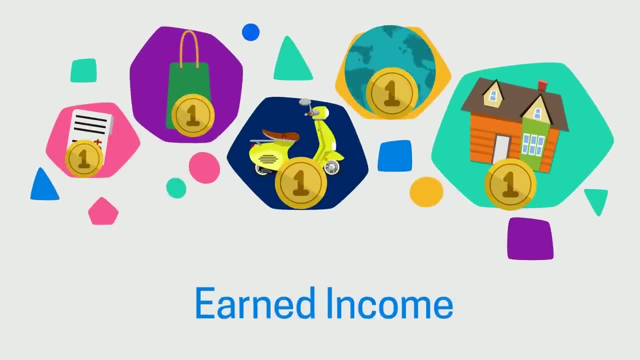 Not having knowledge of how to manage bills and create the distinction between wants and needs can lead to one enduring one hardship after the other. 7. Planning: Everyone needs to know how to plan a lifestyle that is financed by earned income. This includes understanding how to plan for all bills but still ensuring there's enough. 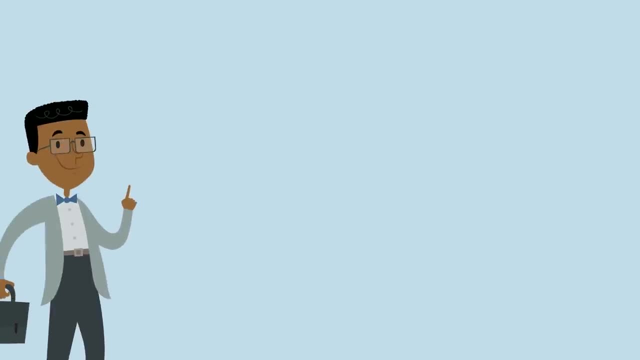 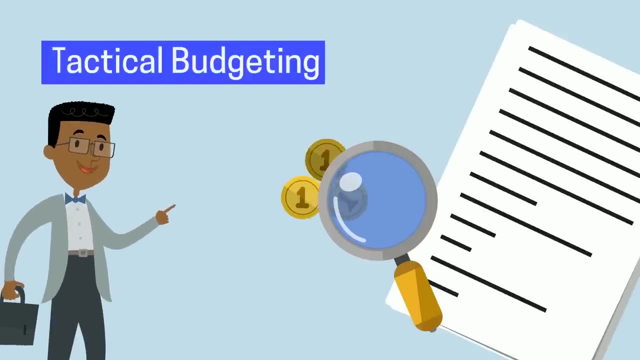 left for necessities such as groceries and savings. But let's face it: as much as budgeting is important, no one really likes tracking every single penny they use. What you can do instead is what we refer to as tactical budgeting. This involves creating budgets and plans over a long period of time. 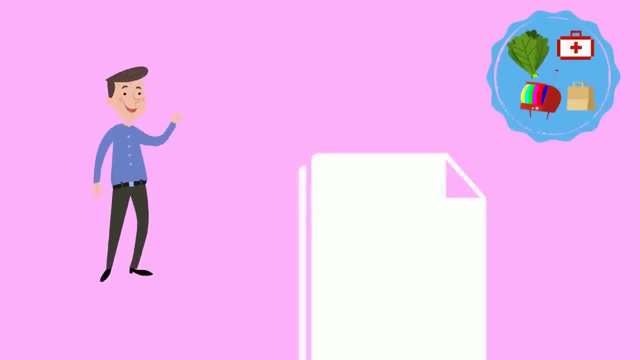 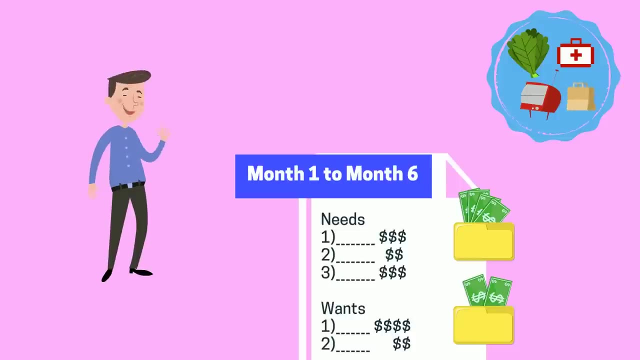 For example, you can identify what you need every month and create a budget with the needs, wants and respective costs over the next month. From the plan created, you can then separate the amounts into different accounts to ensure you don't spend over your budget. 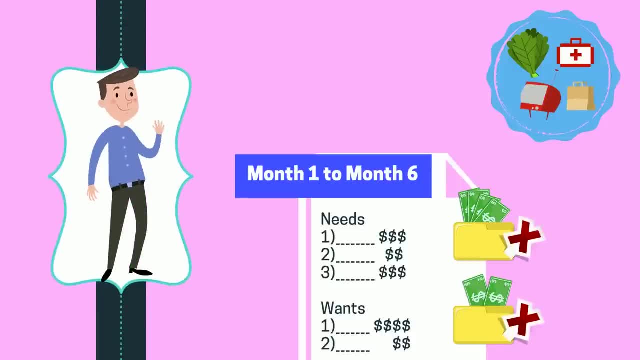 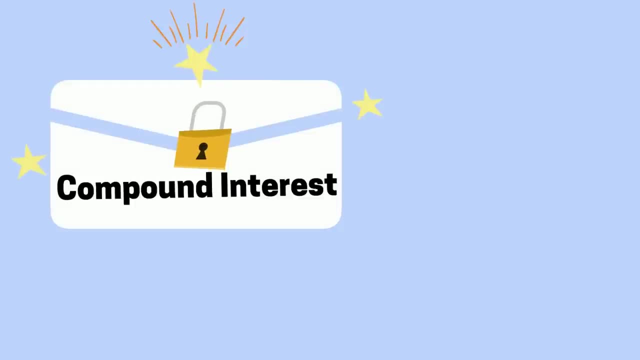 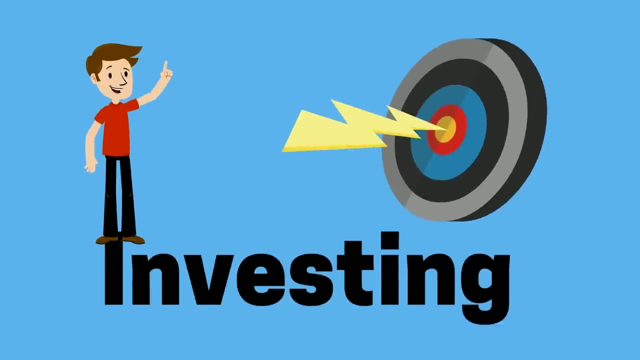 Then occasionally, you can refer to your list to stay on track. 6. Compound Interest. The power of compound interest is possibly the best kept secret. The one thing every young person has an advantage over everyone else is time. While they may not achieve their financial goals instantly, they have an upper hand when. 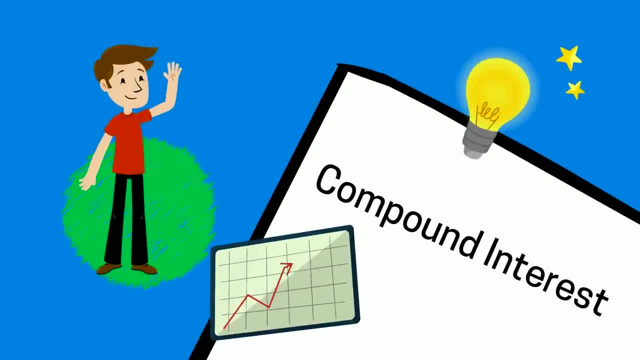 it comes to investing, All they need to do is tap into the powers of compound interest. They're the ones who make the most money. They're the ones who make the most money By setting aside small chunks of money in a high-interest account. young people can. 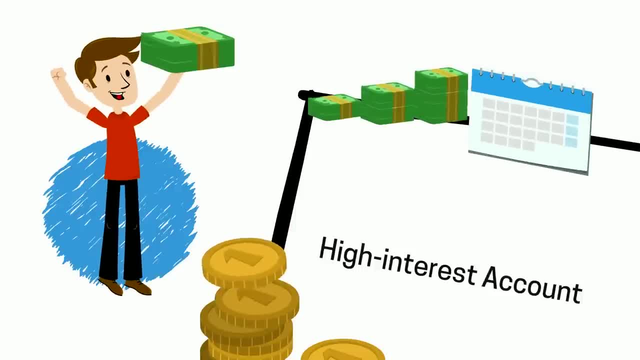 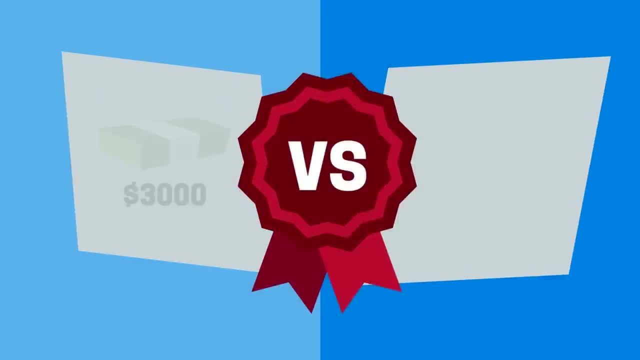 amass great wealth that will compound over and over again through the years. To show you just how important compound interest is, here's a great example. If someone gave you two options, the first choice is $3,000, and the second is a penny. 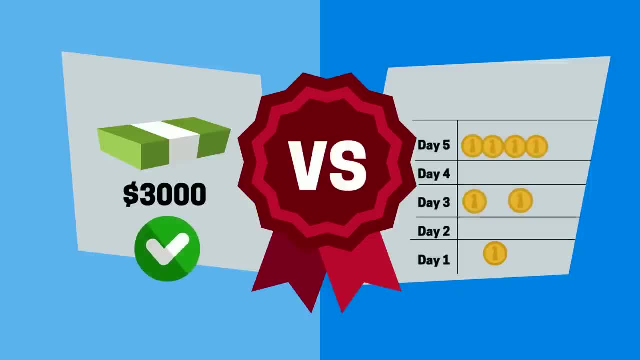 that doubles up in value every other day. Most people would choose the first choice. right? You probably did too, but if you do the math, the second choice would be worth $10 million after 30 days only. If that's the case, then you're probably the one who would choose the second choice. 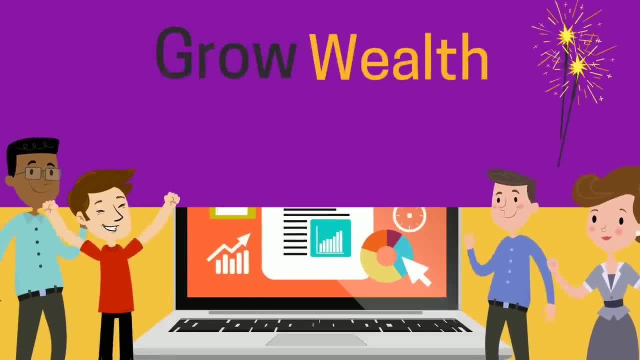 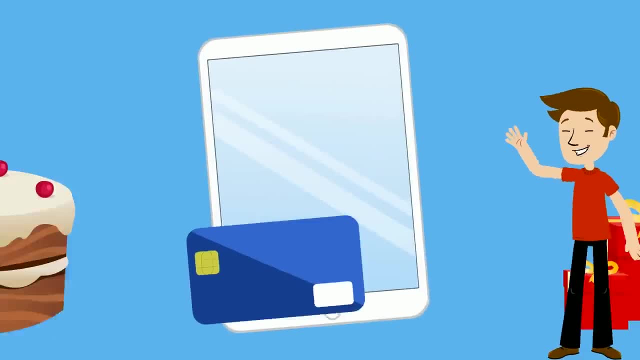 If that's not enough to convince you to start taking advantage of this incredible opportunity to grow your wealth, then I don't know what will be. 5. Secrets of Credit: Most young people, right after getting their first credit cards, end up maxing them out. 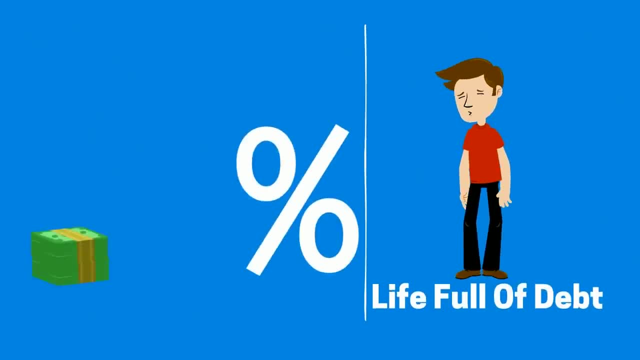 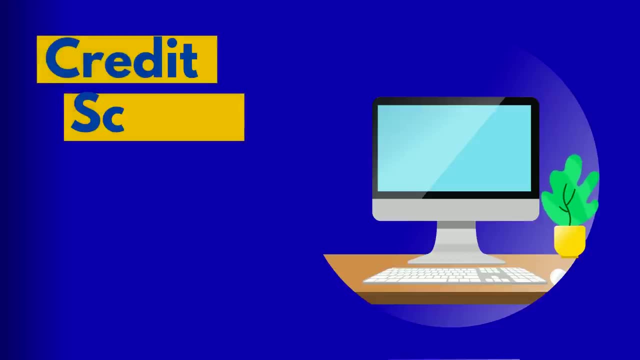 They then end up with a life full of debt where they're forced to pay up huge chunks of interest rates, and in some cases this results in late payments that could adversely affect them. What most people don't know is the importance of credit scores and maintaining a great credit. 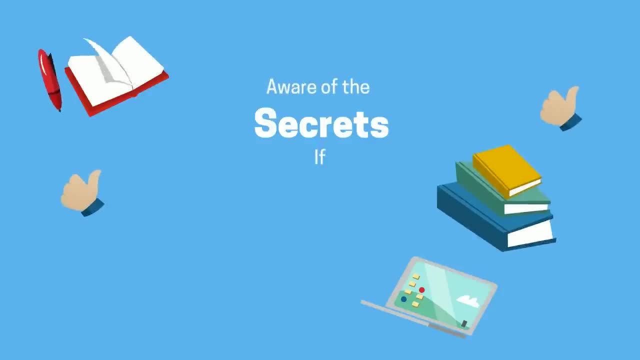 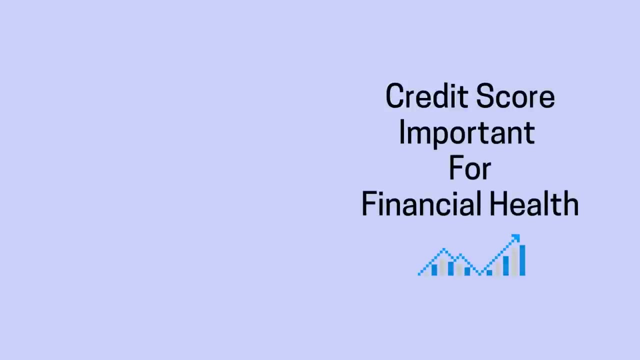 history, But they would probably be aware of the secrets if schools paid more attention to training them on this life skill. Here's what you need to know. Your credit score is one of the most important parts of your financial health and it generally determines your financial position as an adult. 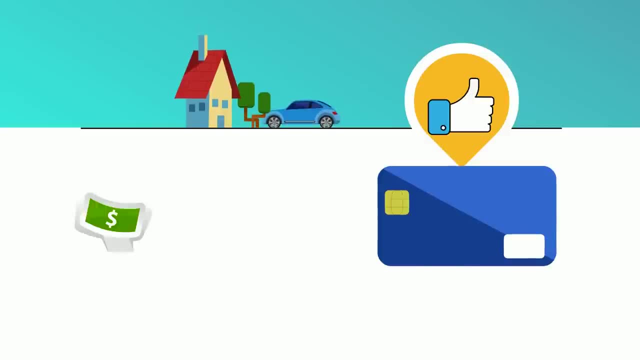 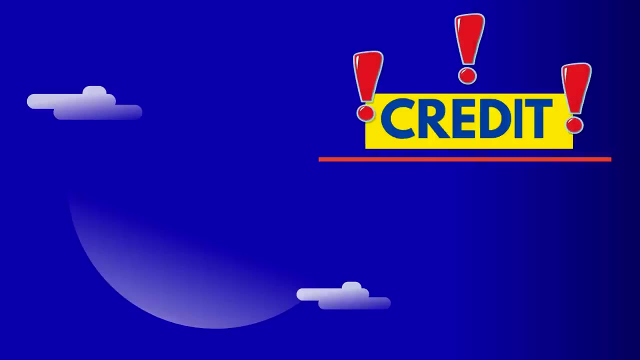 With a proper score, it's a lot easier to purchase a house, get a car, get a business loan and makes it much easier to achieve other milestones in the future. We can no longer ignore the importance of credit. Everyone needs to know how to build credit and have a proper score all the time. 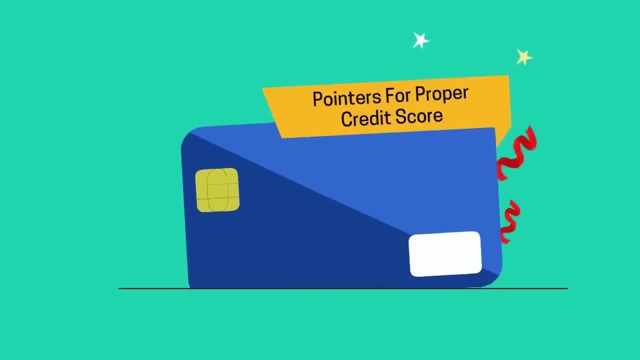 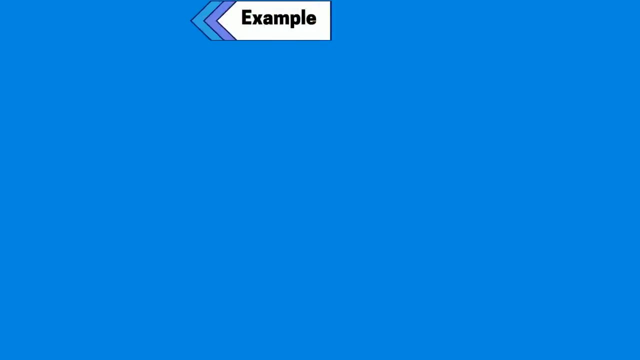 Here are a few pointers on how to achieve this. 1. Get a credit card. Some people think getting a credit card is a mistake, but it is actually quite important in building your credit score. Let me give you a good example. So I have a friend called Kevin. 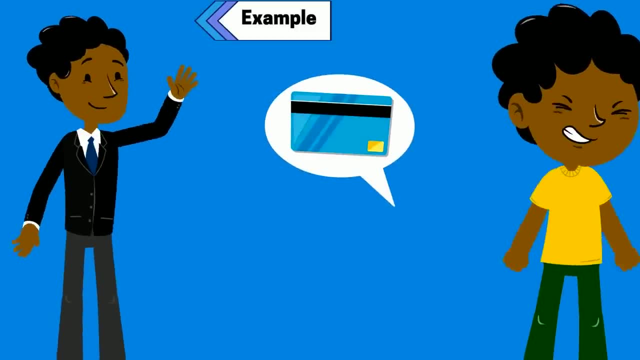 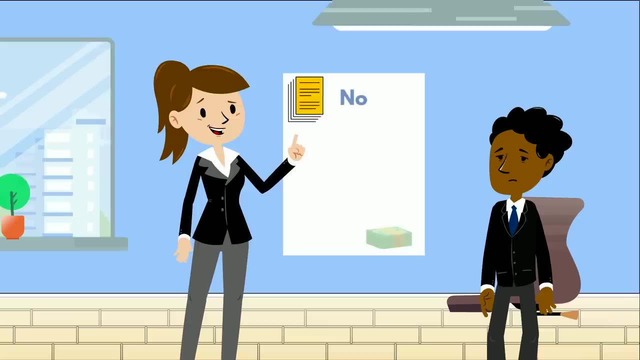 Just like some people, he avoided getting a credit card for most of his young years. after graduating from school. Doesn't sound like a big problem, right? But when he started looking for a home to buy and a car, he couldn't get any loan approved. 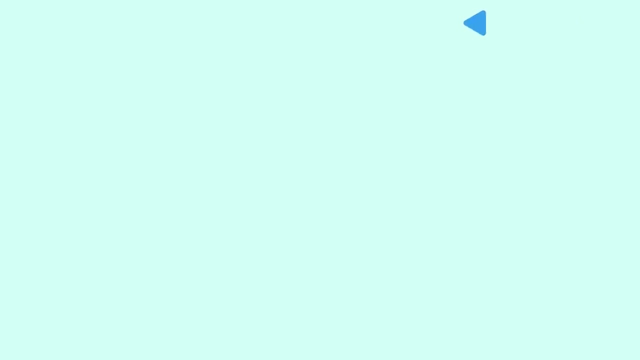 because his credit statement hadn't been established. Here's how it works: When you get a credit card and use it, financial institutions record all your transactions and interest payments. 2. If you're not sure of your efficiency, they'll assign you a score to your name. 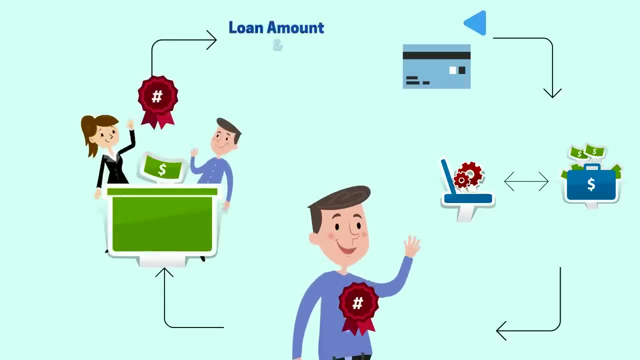 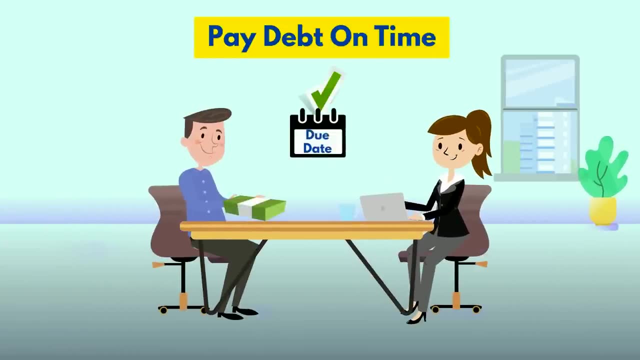 Now, when you go looking for a loan, that score will determine the loan amount you can receive and the interest rate. 2. Always pay your debt in time. There's no other way around this. If money is due today, make sure you pay it today. 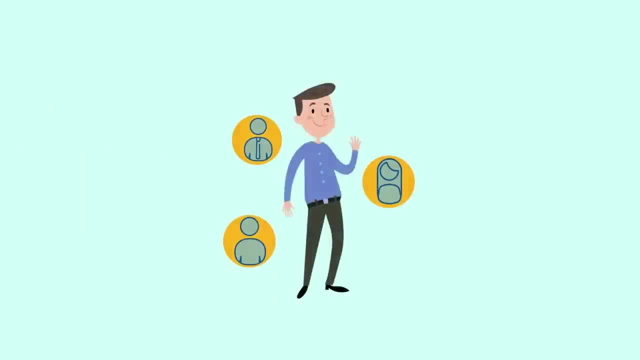 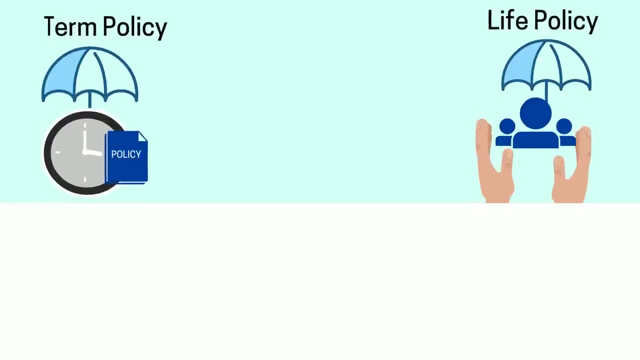 4. Rules of insurance. If there's anyone who is depending on you financially, then you need to get life insurance. This could be your child, spouse or parent. It is better to get a term policy rather than a life one, as you get coverage whenever the 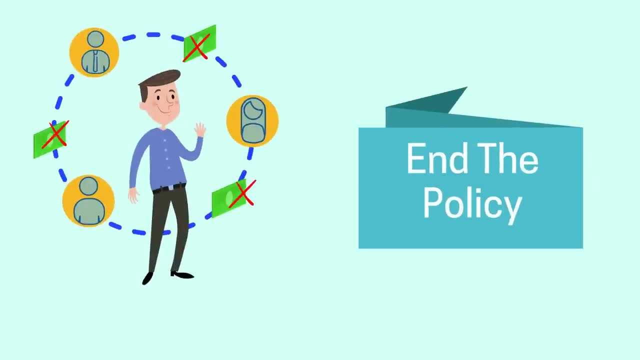 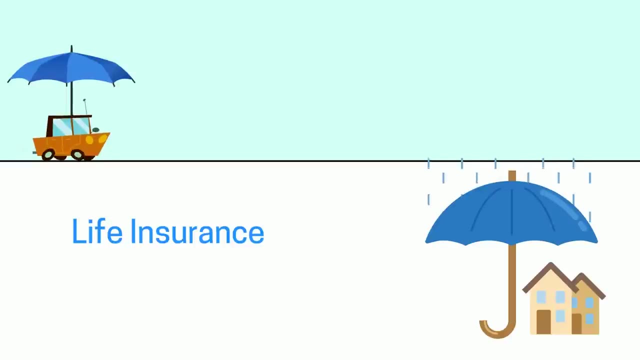 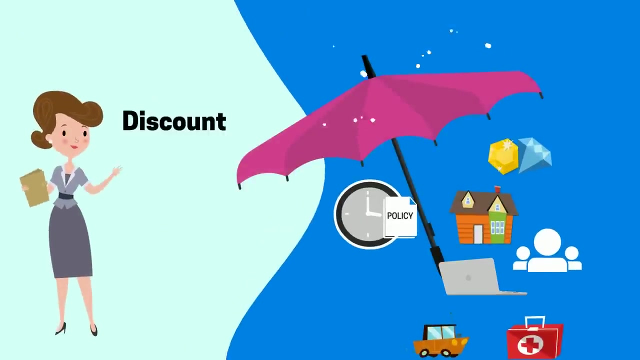 need arises. However, if no one depends on you financially, you need to get life insurance. In addition to life insurance, get insurance for other aspects and assets you own. This includes your car, home, expense assets and health. You can also get umbrella insurance, which covers different policies and guarantees a 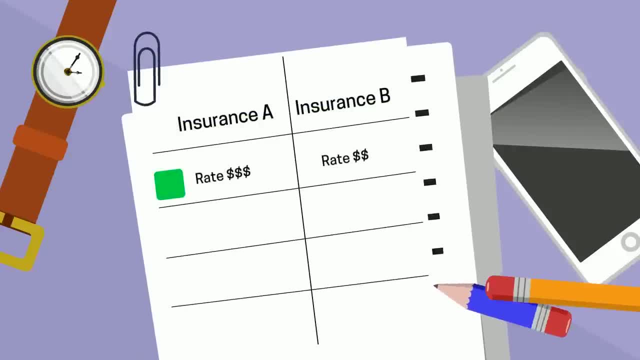 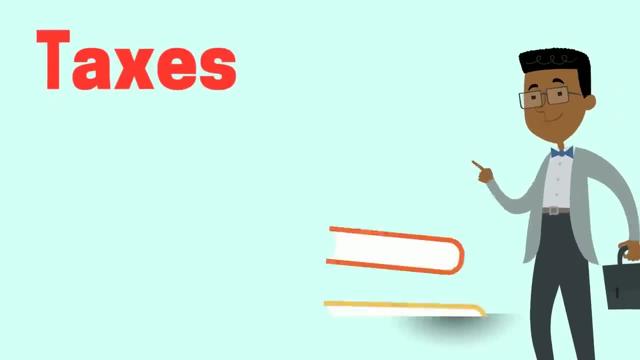 discount if obtained from one insurer. Take your time to get different rates and the features available before choosing a company to insure with. 3. Taxes: Taxes are such a broad topic that is hardly ever discussed in school. It's important to understand how they work. 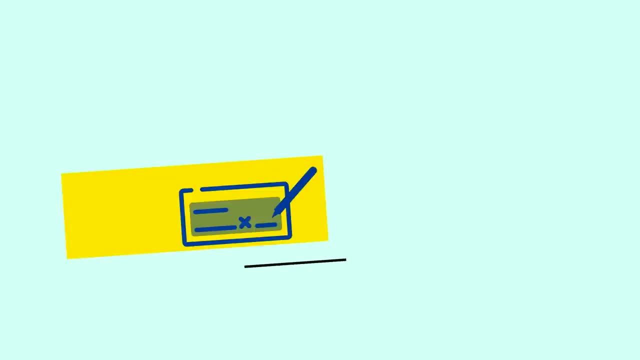 If you want to be on the right side of the law, before you get your first paycheck or make any sales from your business, learn how to calculate the tax rate and find out how much money you'll be left with. This will help you determine whether a job offer will meet your financial needs and what. 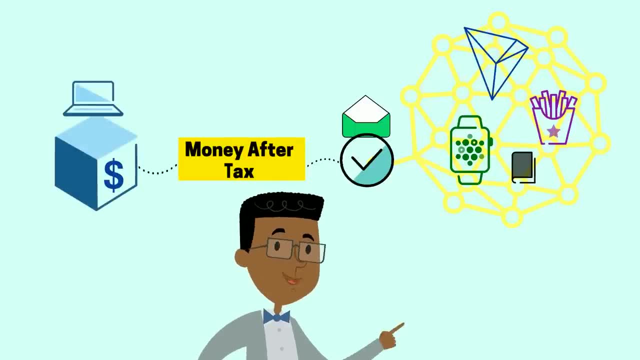 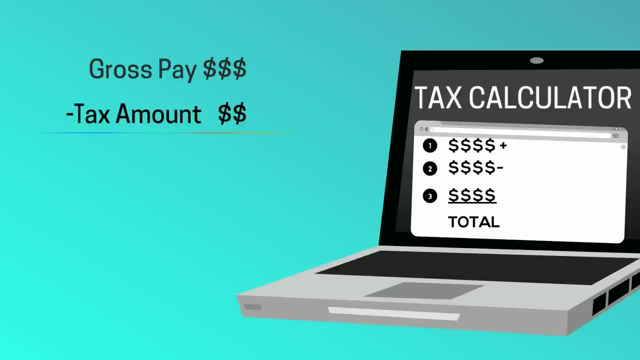 the appropriate pricing strategy for your products or services will be. Luckily, there are plenty of online calculators that will do the dirty work for you. They will show you the gross pay, the amount payable in tax and the amount left in your account, also known as the take-home pay. For example, a salary of $35,000 a year in Manhattan, New York. If you want to be on the right side of the law before you get your first paycheck or make any sales from your business, learn how to calculate the tax rate and find out. 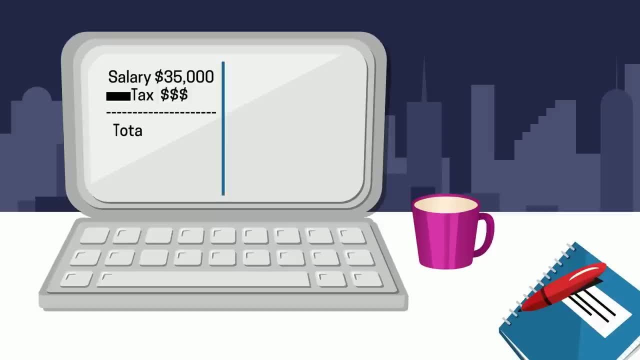 how much money you'll be left with. This will help you determine whether a job offer will meet your financial needs and what the appropriate pricing strategy for your products or services will be. This will help you determine whether a job offer will meet your financial needs and. 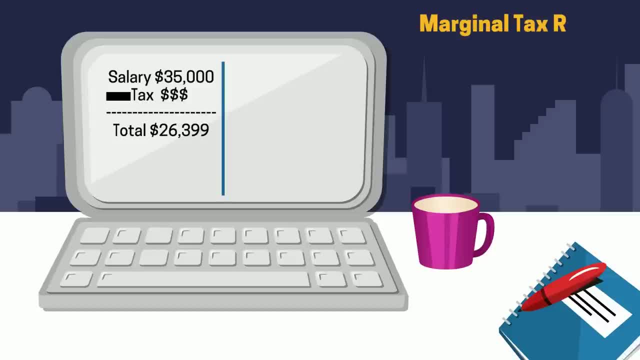 what the appropriate pricing strategy for your products or services will be. Also pay attention to the marginal tax rate that affects your raise. For example, a raise of $35,000 to $41,000 a year won't give you an extra $500 a month. 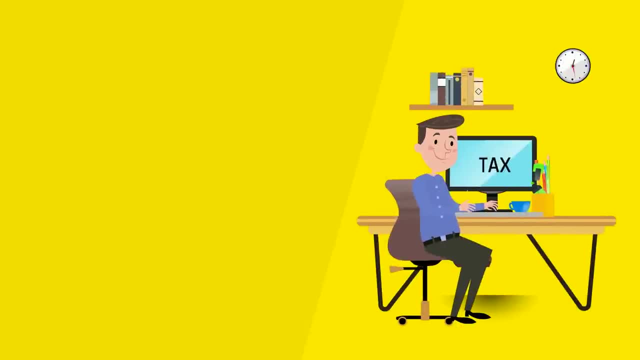 but $345.. Make a habit of preparing your tax returns yourself. There's a lot of misinformation and bad advice out there. Be careful. 2. Guard your health. A hospital visit for an injury like a fractured knee can cost thousands of dollars. 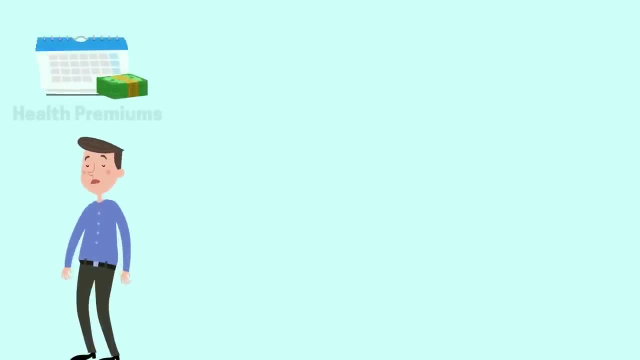 If you're finding it hard to meet your monthly premiums, then what will happen if you end up in the emergency room? You may end up having to borrow money to pay for your medical bills, burdening other people who had plans with their money. Doesn't sound fair, right? If you don't have a medical cover, get one ASAP. Also, taking care of your health can end up saving you a lot of money. This involves eating the right foods, maintaining a healthy weight, regularly exercising, not. 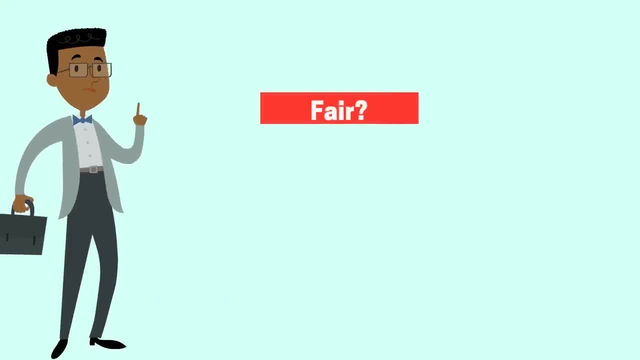 consuming alcohol and other additives excessively. You don't want to be sorry, so guard your health through the day. You may end up having to borrow money to pay for your medical bills. burdening other people who had plans with their money Doesn't sound fair right. 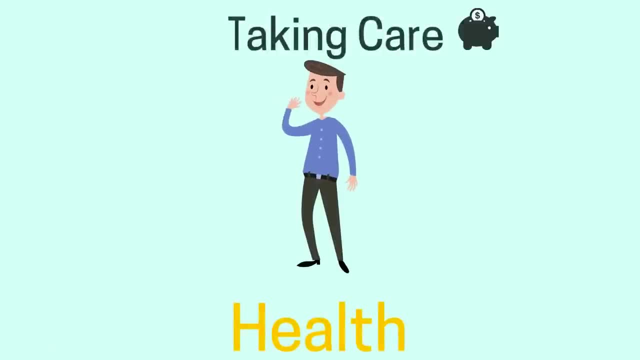 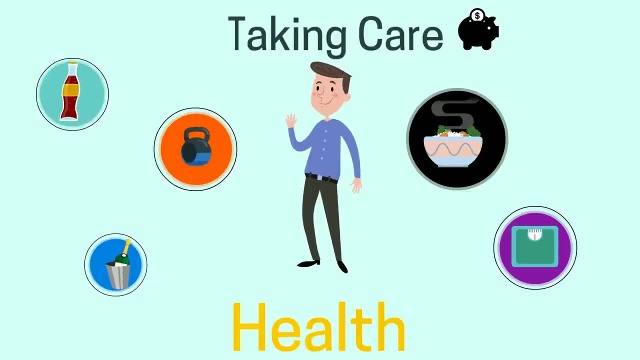 If you don't have a medical cover, get one ASAP. Also, taking care of your health can end up saving you a lot of money. This involves eating the right foods, maintaining a healthy weight, regularly exercising, not consuming alcohol and other additives excessively. 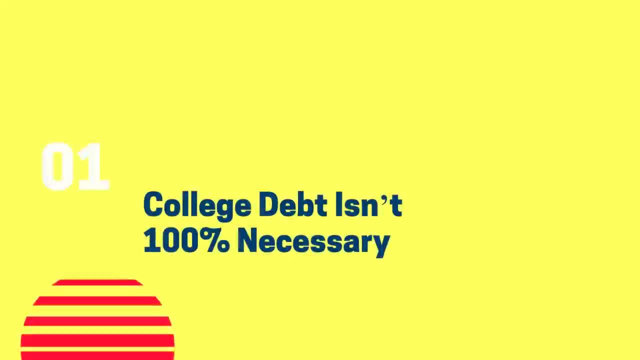 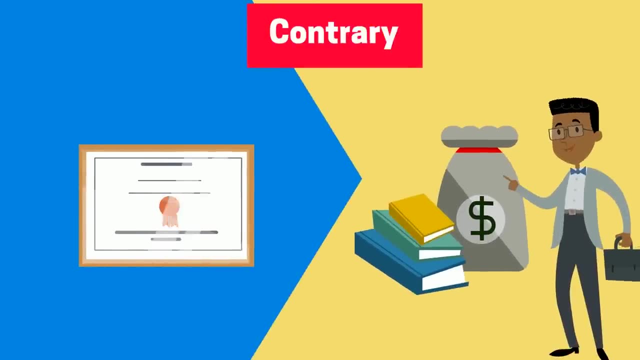 You don't want to be sorry, so guard your health today. 1. College debt isn't 100% necessary. Contrary to what everyone believes, that student loans go hand in hand with a college degree, you actually don't need to get one to achieve.